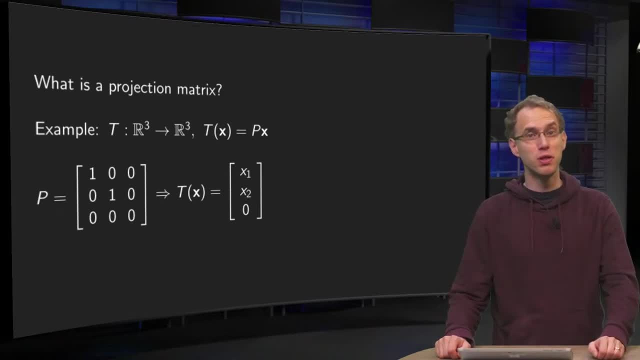 You have learned how you can compute the projection of a vector on a subspace. Such a projection is an example of a linear transformation, So this projection is implemented by a matrix. But how can we find this projection matrix? That is what you will learn in this video. 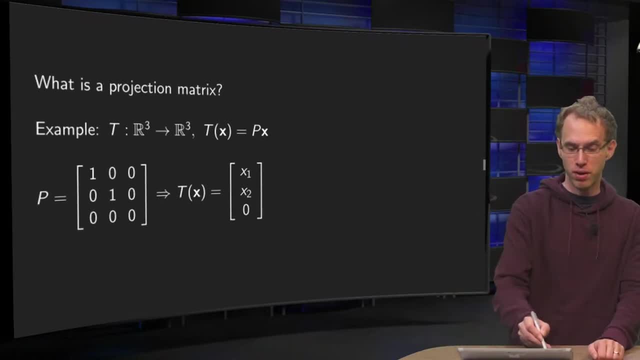 You have seen an example already: If we have a transformation from R3 to R3, Tx equals Px. where P is a matrix, Then we have seen this matrix P with 1's here and here and all of our 0's. 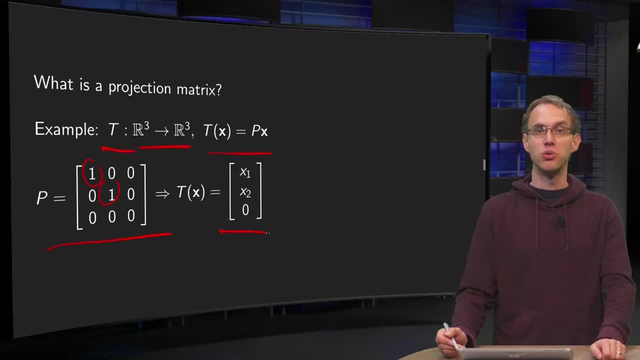 And now, if you compute P times x, you get the vector x1, x2, 0. So what this transformation does? it makes the last component 0. Which means that it is basically projecting on the x1, x2 plane. 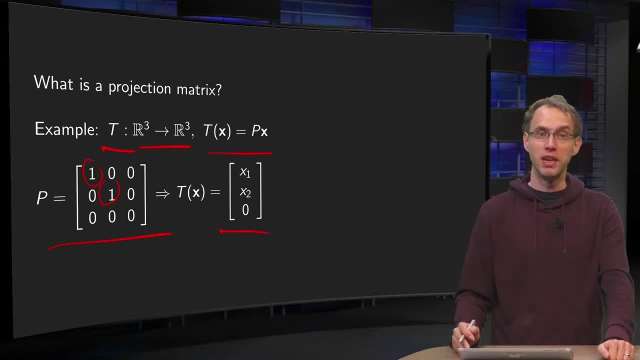 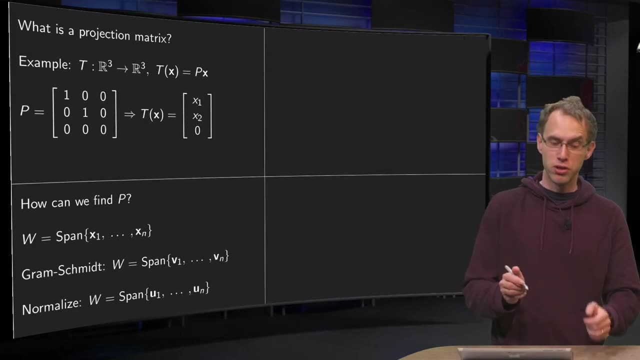 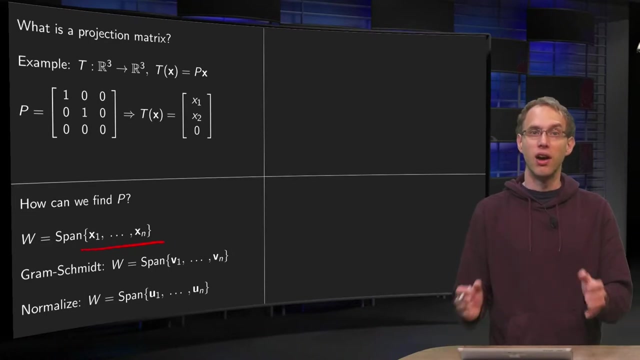 So here we have seen already an example Of a projection matrix. But how can we find such a projection matrix in general If we have given some span of x1 up till xn Where x1 up till xn is some basis, How can we find our P in that case? 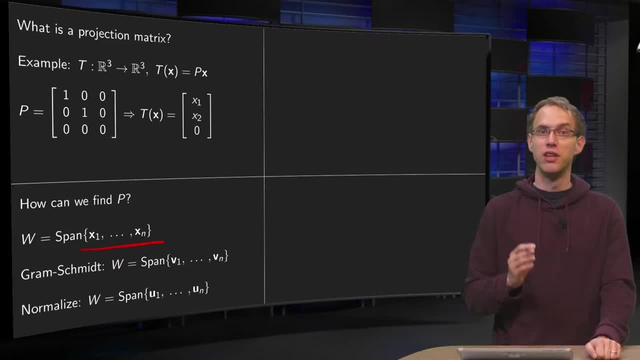 Well, first of all, we are going to build an orthogonal basis. You know how to do that. We use Gram-Schmidt, And then we find our v1 up till vn, An orthogonal basis For our w. Then next step, we are going to normalize. 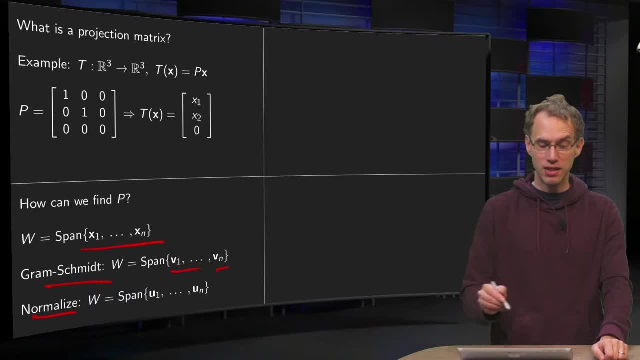 That's easy. You just divide all v's by their lengths and you get u1 up till un. So now you have an orthonormal basis for w. Usually the u1 up till un will look ugly Because you have normalized them. 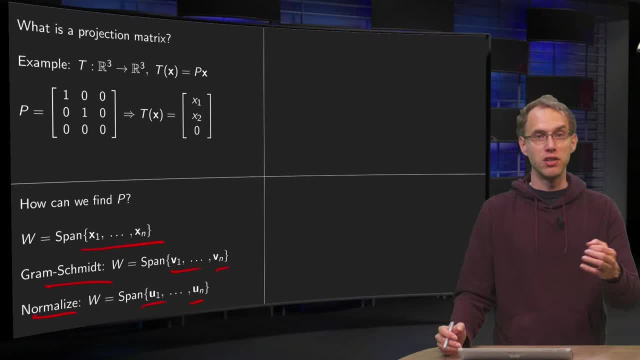 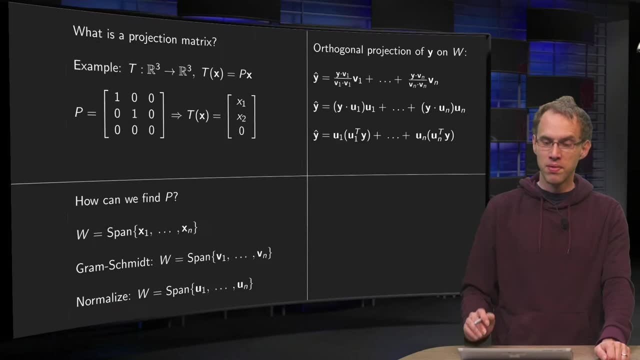 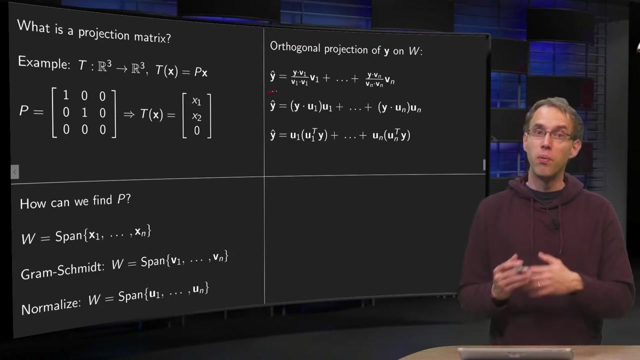 So their lengths are 1. now, however, the vectors themselves often involve some square roots. Then then We know the projection formula y hat. So if you want to project y onto w, then you have to use an orthogonal basis or an orthonormal. 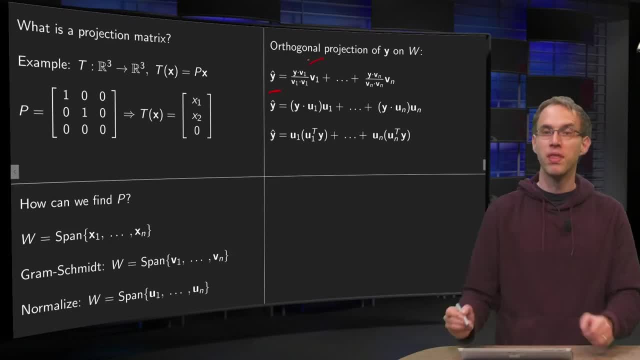 basis. And here we have our projection formula: y in v1 divided by v1 in v1 times v1, up till y in vn in vn times vn. Now you can use your orthogonal basis. You can use your orthogonal basis, So you do this. 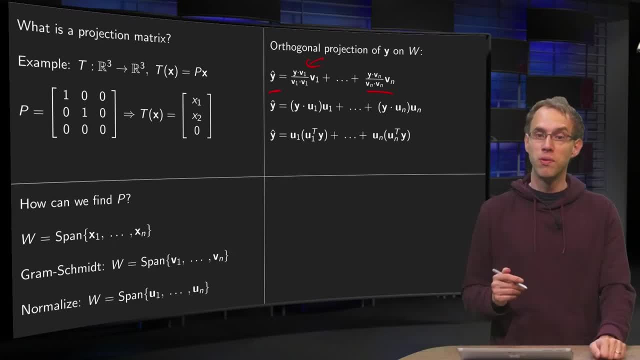 You use the u1, u2 instead of v1, v2.. And the advantage is that you get the u1 in u1 over here and that one drops out Because you've normalized. So u1 in u1 is 1.. So then our projection formula looks like this: 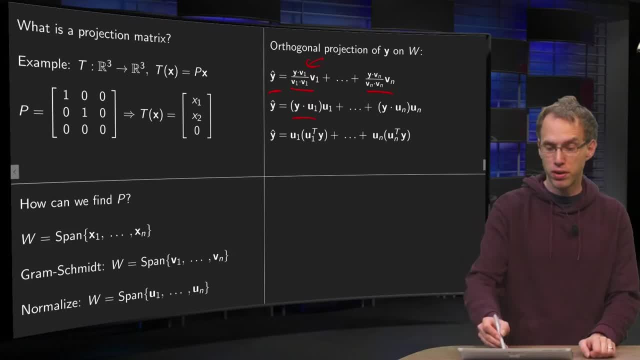 We are only left with y in u1 times u1, up till y in u n times u n. And now we are going to rewrite this formula in order to get it in the form y hat over y hat equals some matrix times y. So we need several steps for that. what do we do? 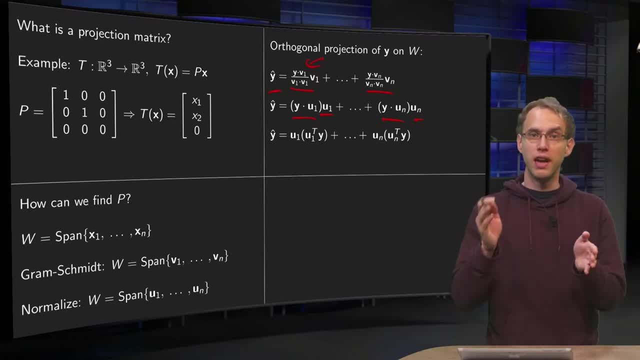 First of all, you can always rewrite your inner product u in v as u transpose times v as a matrix product. So that's what we do with all our inner product. A y in u1 can also be rewritten as u1 transpose times y as normal matrix product. 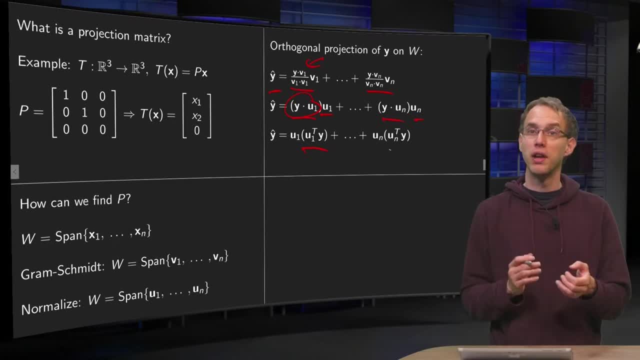 You do that with all of them until the last one. u? n transpose times y, And you have to multiply them, of course, by u1, up till u? n. Ok, there we are, and what you see now is that over here you have vector times, scalar plus. 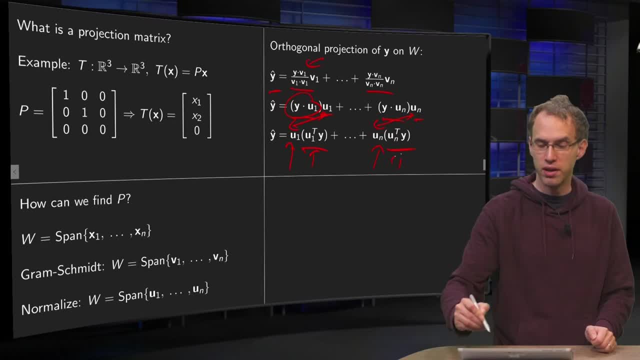 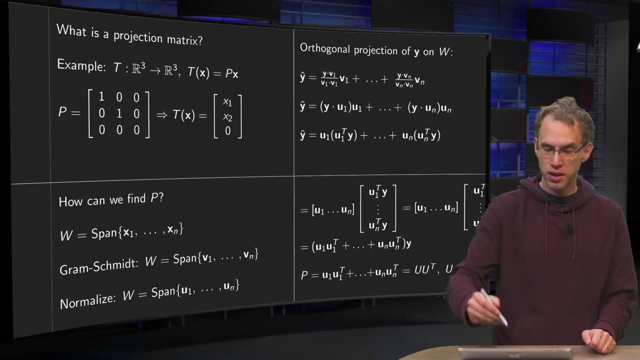 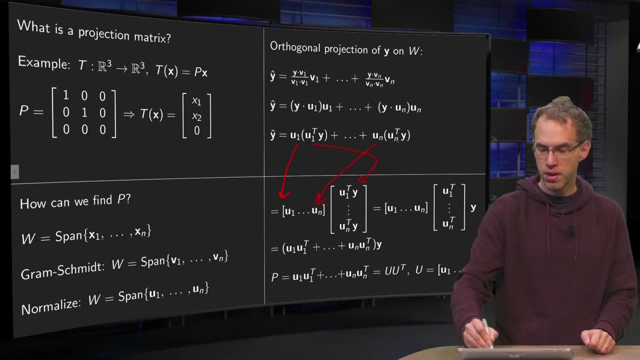 vector times scalar plus vector times scalar plus vector times scalar. So it means that you can write your y hat as a matrix times a vector as follows: You put all the vectors in a matrix and all the scalars in a vector and then you still. 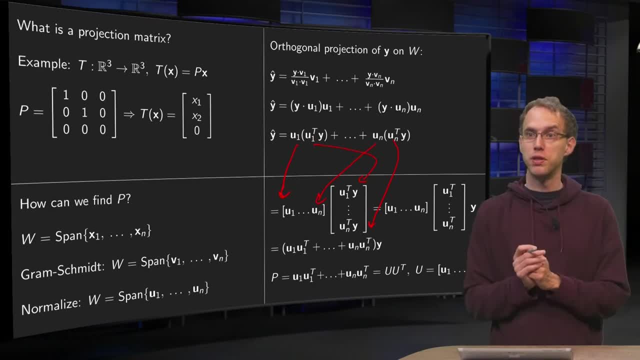 have your y hat, because if you write this out, what this means is this product. if you compute matrix times vector, you get first component times, first vector, and so on and so on. Going back is easier to see that this indeed holds. Then we are going to take the next step. you see, in the vector y is everywhere, so we can. 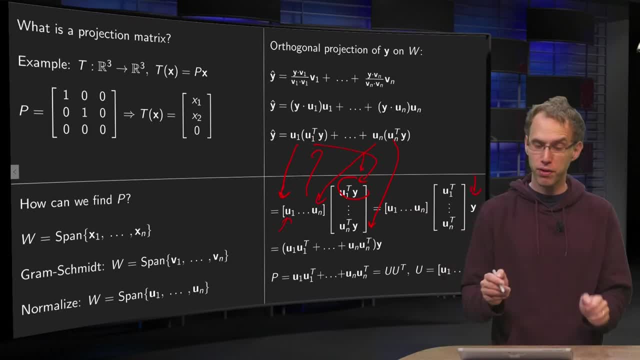 take the y out, Y is coming here. So now you have your y hat equals matrix with u1 up till u n times a matrix with u1 transpose up till u n transpose. So you already see that your y hat equals matrix u times u transpose times y.